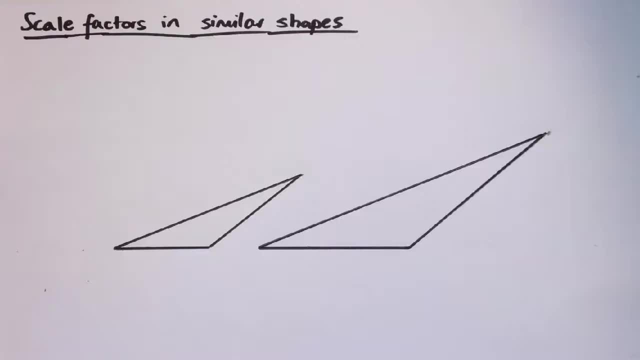 So scale factors are really relevant to similar shapes, and what I mean by similar shapes are, you know, shapes which are essentially the same shape but of different sizes. So one of these is really just an enlargement of the other one. This is just a larger version. 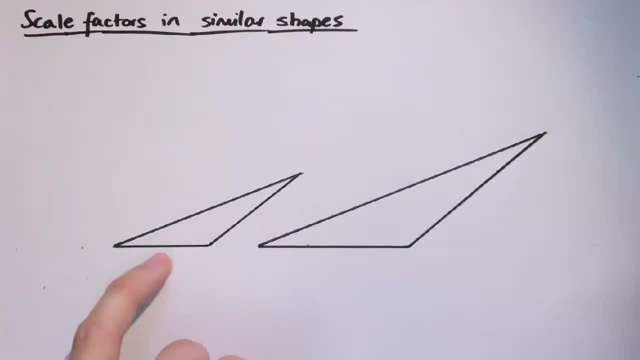 of this one and vice versa. This one is just a smaller version of this one, So let's put some measurements on here, and these measurements aren't exact, but they'll do for our purposes. So if this is just an enlargement of this one, then there's going to be a scale factor. 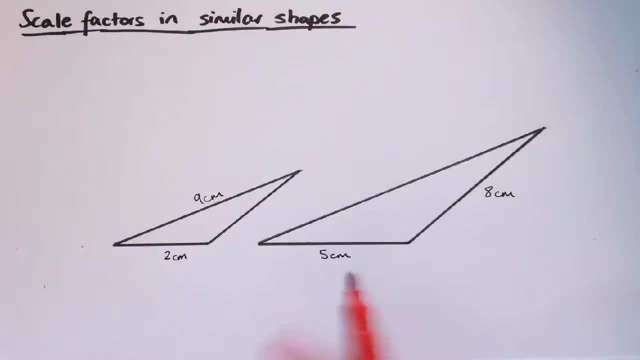 which links lengths in this larger shape to lengths in the smaller one. And if we've got two corresponding lengths- as we have here, we've got the 2cm and the 5cm- we can think of a scale factor taking us from the smaller shape to the larger shape. So the scale factor, 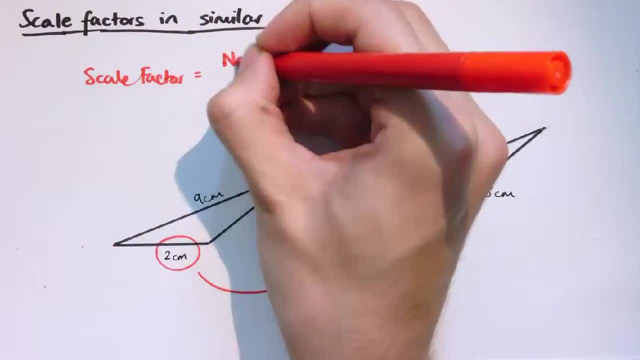 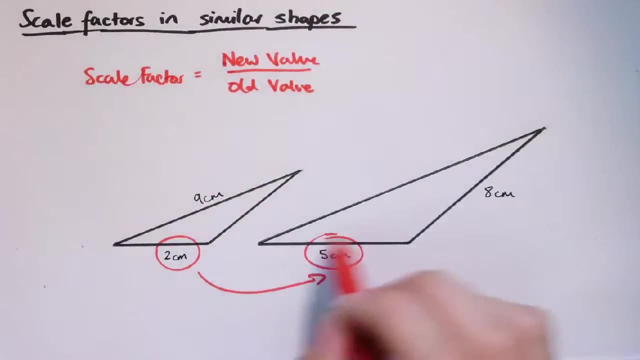 as we know from previous videos, is the new value divided by the old value, and here we're thinking of the new value as 5cm and the old value as 2cm. so the scale factor is 5 over 2, or 2.5.. And once you've worked out the scale factor, because the shapes are- 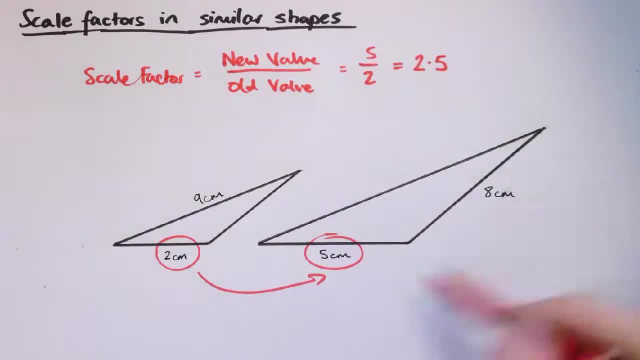 similar, then every length in here is just 2.5 times as big as the corresponding length over here. So let's say, Let's say I wanted to work out the length of this side x. Well, I could just apply. 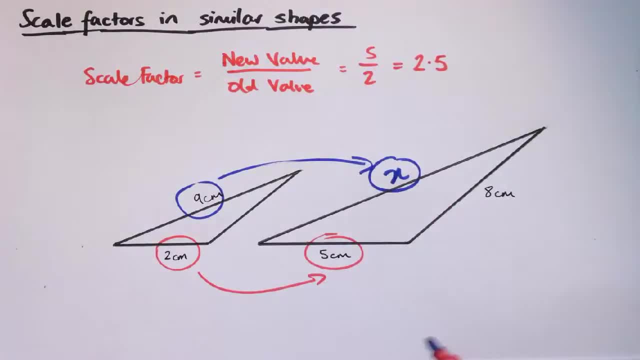 that same scale factor from here to here, and I could say: well, x is equal to 9 times 2.5,, which is 22.5.. So this x here would be 22.5cm. To find this distance, y, which is: 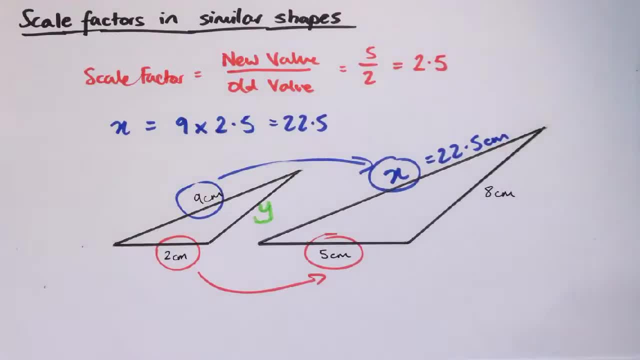 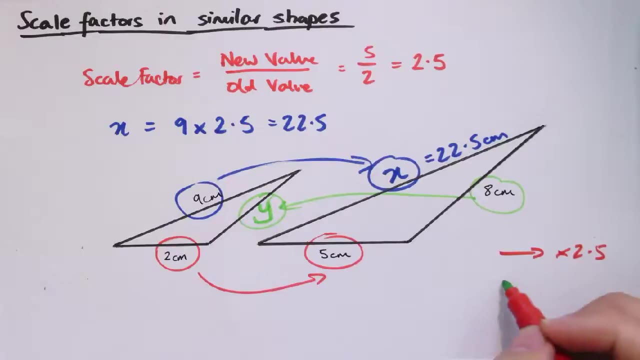 22.5cm. Well, we want to go back from here to here this time. so if the scale factor going in this direction is 2.5, or multiplying by 2.5, to undo that we would do divided by 2.5, or. 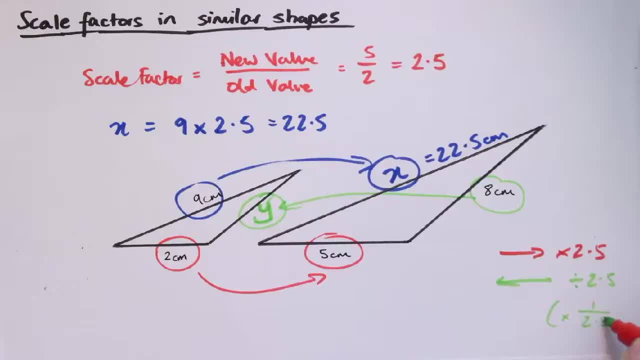 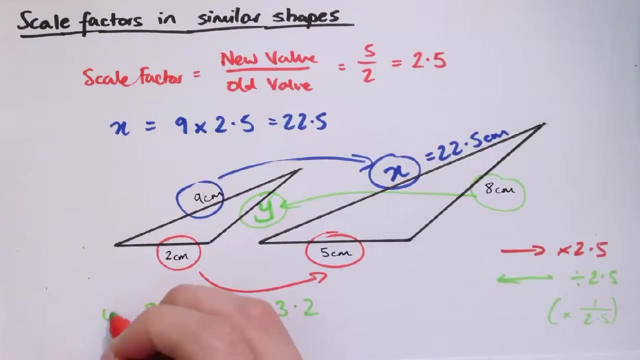 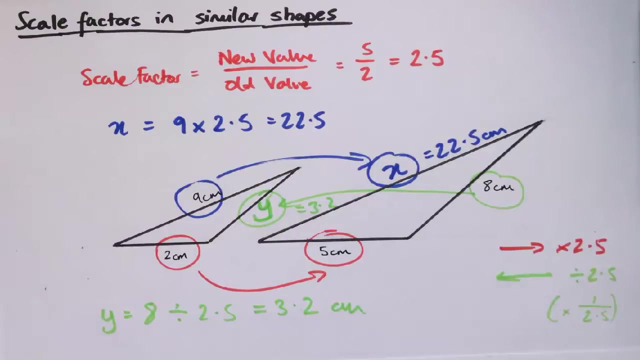 you could equivalent, say, times 1 divided by 2.5. So we would do 8cm divided by 2.5, which would give us 3.2 centimetres for y. You could, if you like, have said: okay, well. 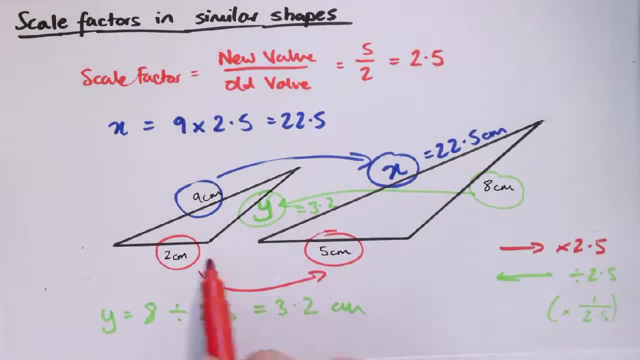 you know, work out the scale factor separately and say, okay, if we're just going the other direction, the scale factor, rather than being 5 over 2, would be 2 over 5.. So that's actually the same as saying that's exactly the same as saying 8. 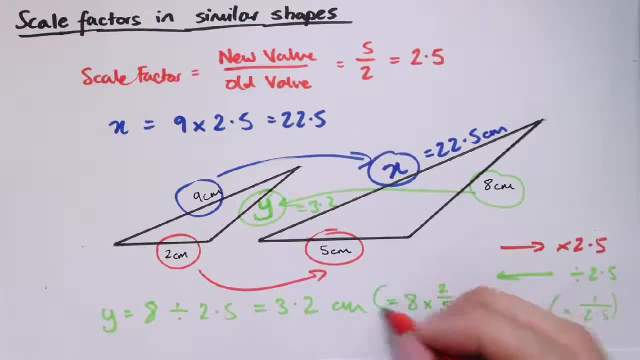 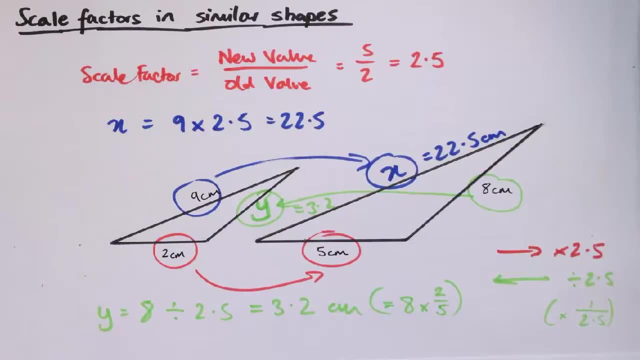 times 2 fifths, Or we can just use the reverse scale factor. whichever you prefer. You need to be able to be sort of fluent in doing it. both ways really, but powerful idea because if we have similar shapes and we know the scale factor, we can find. 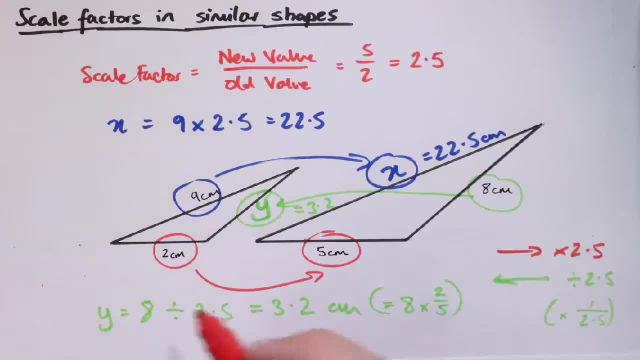 missing lengths. It doesn't apply just to lengths of sides, it could be you know the length of the whole perimeter. say So, for example, on the right here we've got the perimeter is, and the perimeter of this one is 5 plus 8 plus 22.5. 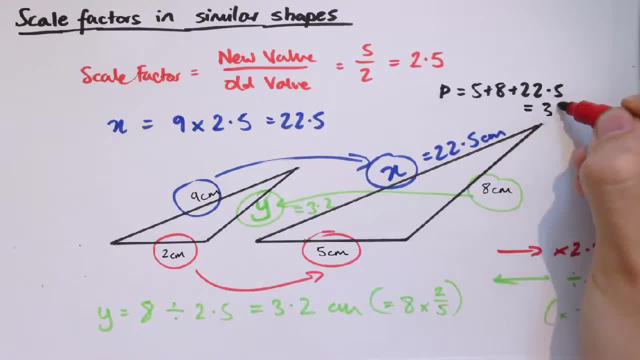 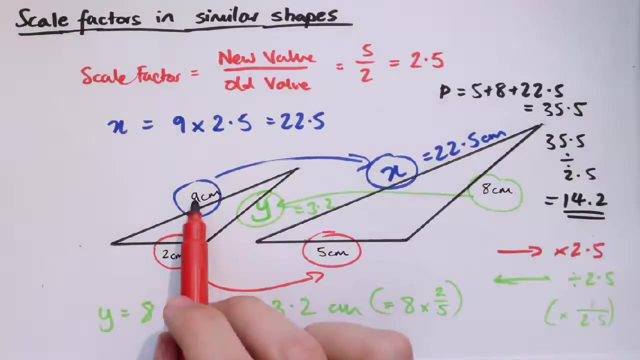 that's 35.5. and if we take 35.5 and divide it by 2.5 then we get 14.2, which is the perimeter over here. 9 plus 2 plus 3.2 is 14.2.. If I had a squiggly line in here that was length. 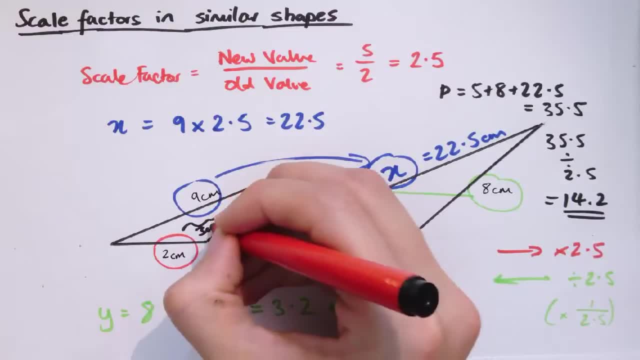 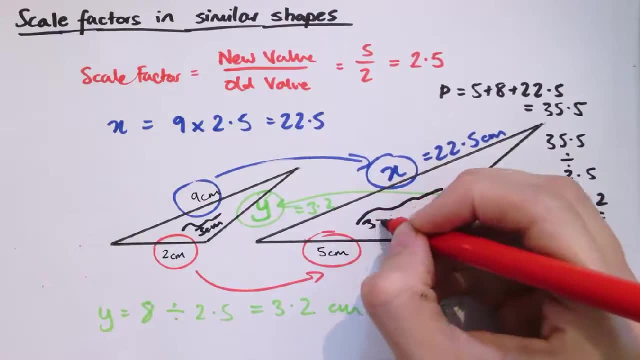 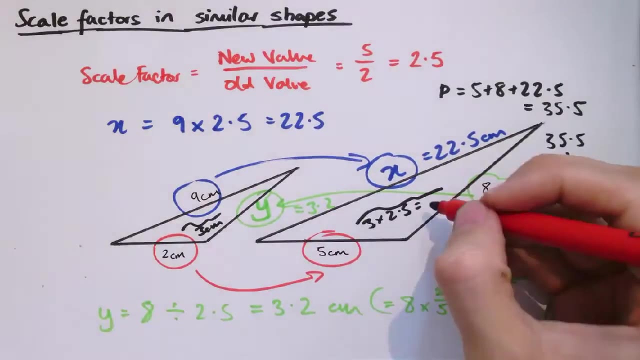 you know 3 centimeters, and I had a. now it would have to be an exactly corresponding, similar squiggly line in here, but its length would be 3 times 2.5 or 7.5. so any corresponding length in the other shape is scaled up by the same. 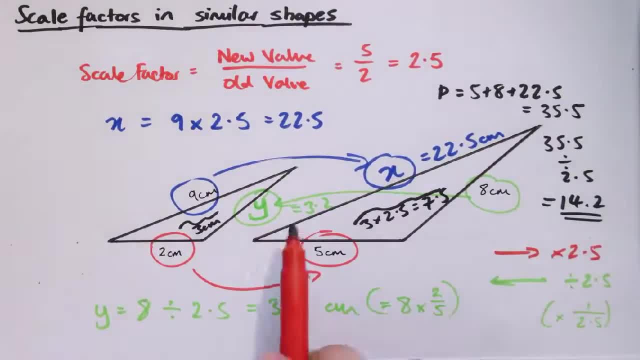 scale factor. It doesn't apply to areas. we've got a different result for areas. The area isn't just scaled up by 2.5.. but any length that corresponds does scale up in exactly the same way by that scale factor, the length. And in fact, because it 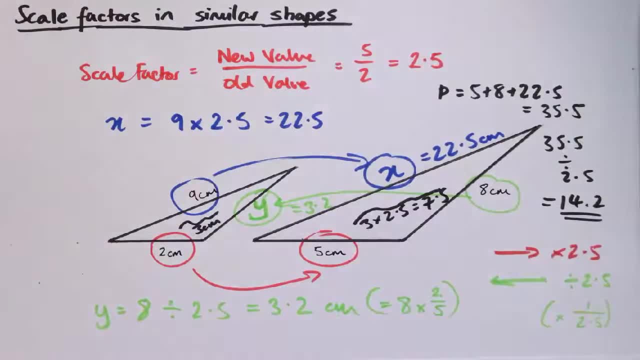 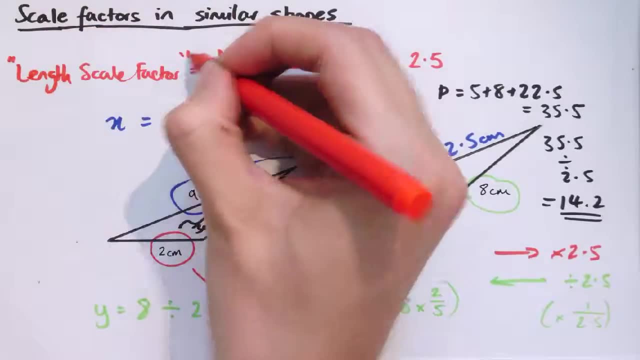 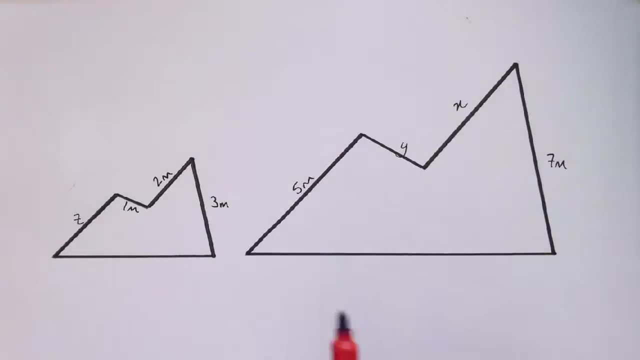 only really applies to lengths and not to areas or volumes and things like that. we might sometimes even refer to it as the length scale factor. Here's another example, then. So, supposing these two shapes are similar, they look pretty similar. I haven't drawn them absolutely exactly, but if we assume we're going to draw them exactly the same, 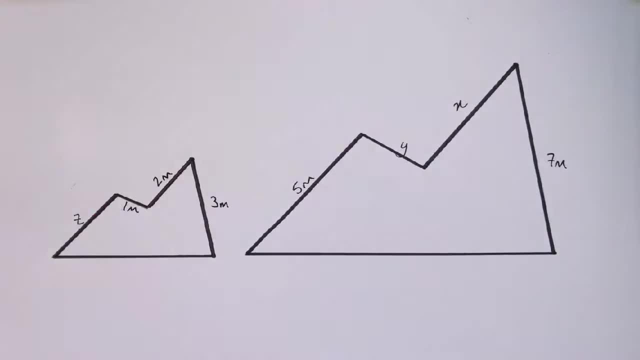 or the angles are exactly the same, so these two are just similar. there'll be a constant scale factor that goes from one to the other. So we've got to find the pair of values that match up where we have both the values here. so we've got 3 meters here and 7 meters here. so the scale 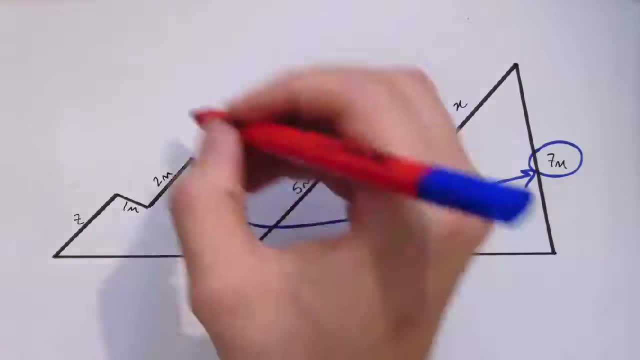 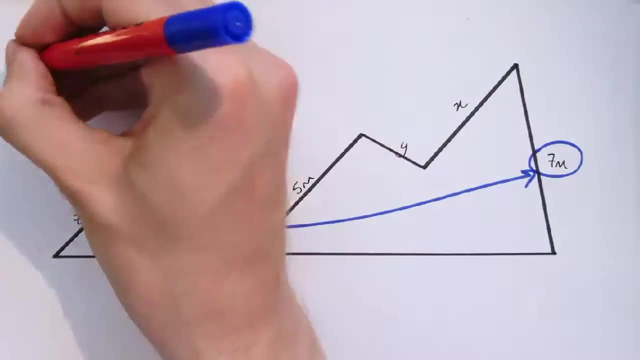 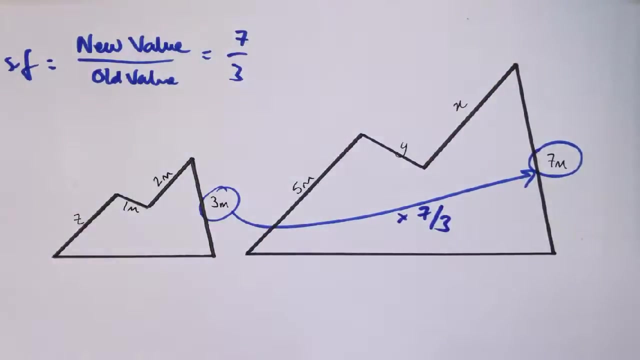 factors are going in this direction: new value over old value for the scale factor, for the length scale factor, that's 7 over 3. so there's my scale factor of 7 over 3.. If I'm going in the other direction then we could divide by 7 over. 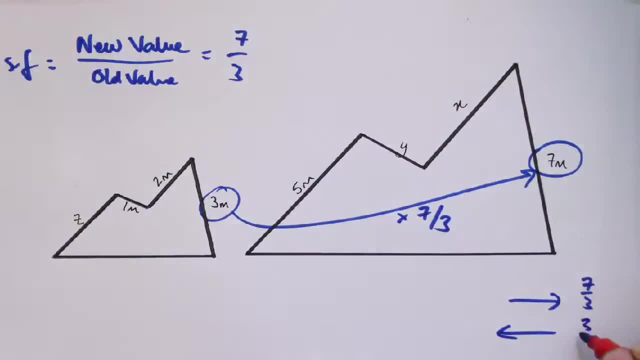 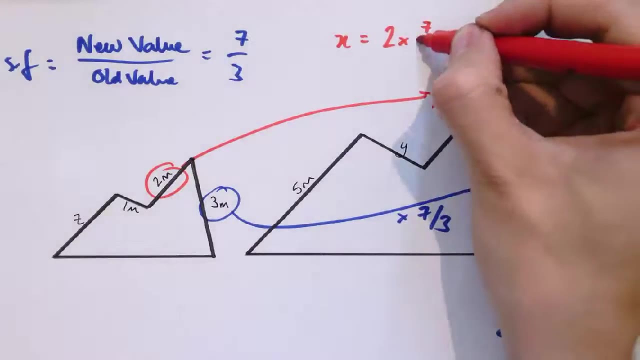 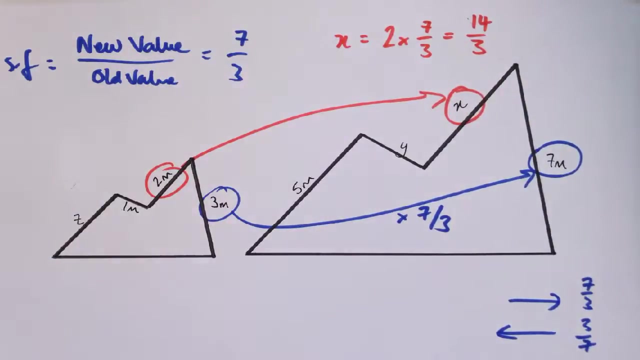 3, or we could say it's a scale factor of times 3 over 7.. So let's use this to find x. then. So x corresponds to this side here. So x is 2 times that same scale factor of 7 over 3, so that gives us 14 over 3.. Leaving your answers as these sorts of fractions is. 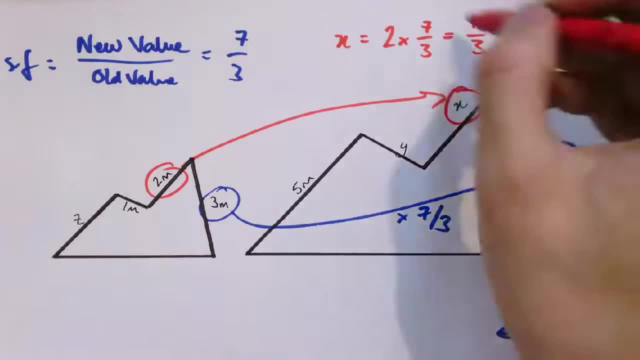 usually fine, by the way, You might want to. you know you could also say, oh, it's 4 and 2 thirds, so you could round that off if you wanted to 4.67 or something, But usually 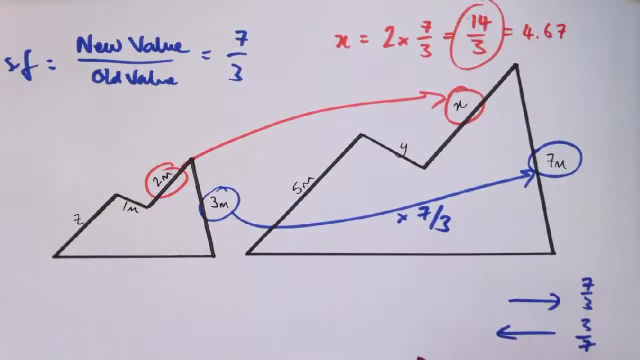 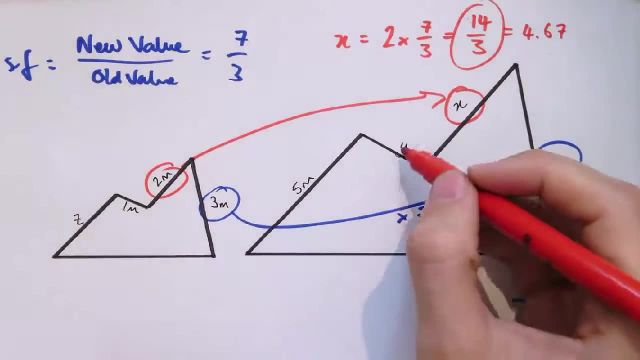 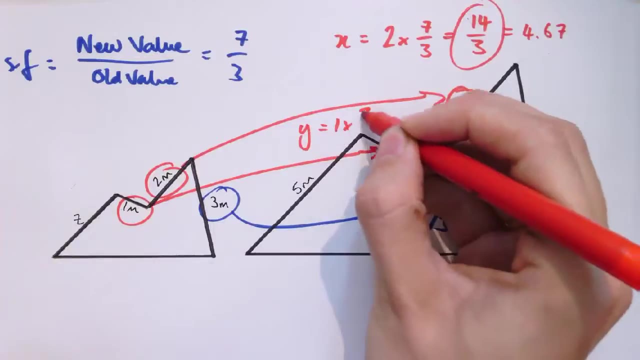 better to leave it as a nice exact value there, so we don't have to round anything off y again. well, y just corresponds to 1 metre over here, So that's easier. That's y is just 1 times 7 over 3, so y is 7 over 3 metres. And for: 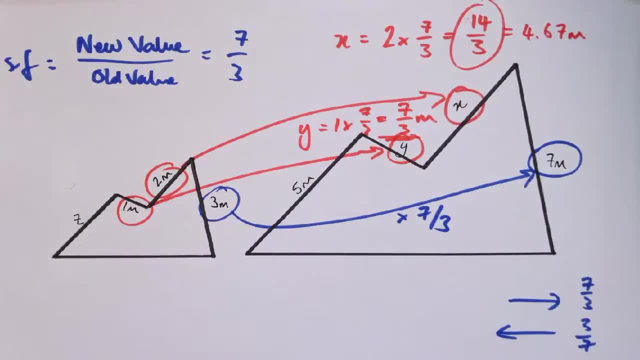 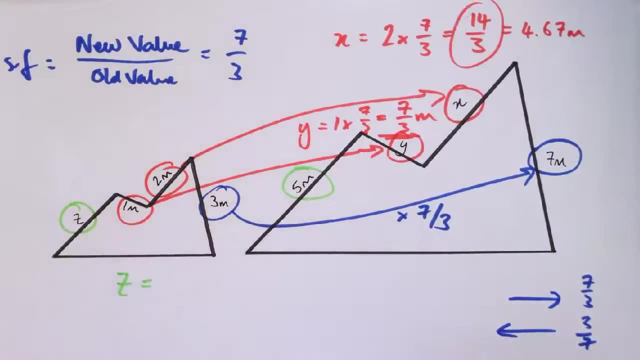 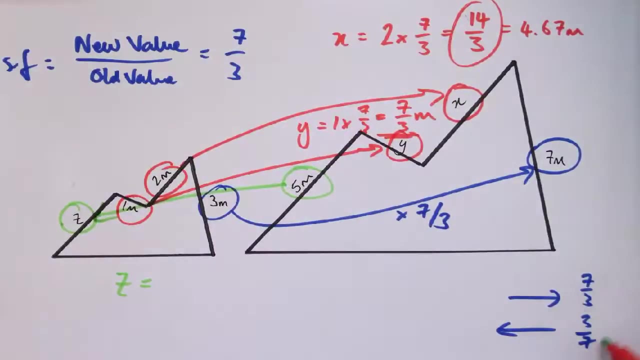 z, we're going back in the opposite direction. this time z corresponds to 5, so either divide by that scale factor of 7 thirds or just multiply by the equivalent scale factor in the opposite direction of 3 sevenths. So z is 5 times 3 sevenths. 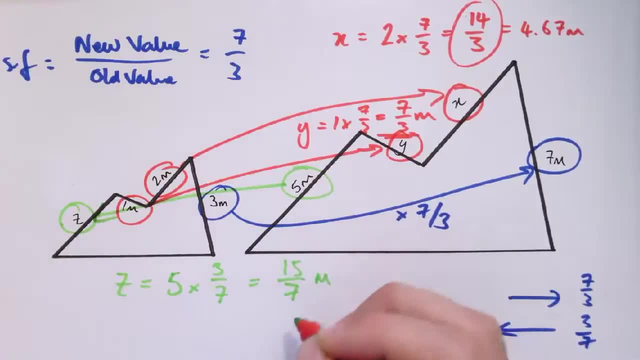 Which is 15, over 7 metres, which is 2 and a bit metres. If you really wanted to, you could write that, as you know, 2.14 metres. That's rounded off a little bit because sevenths aren't exact. So but there we go. Really, I don't want to show you much about the rounding. 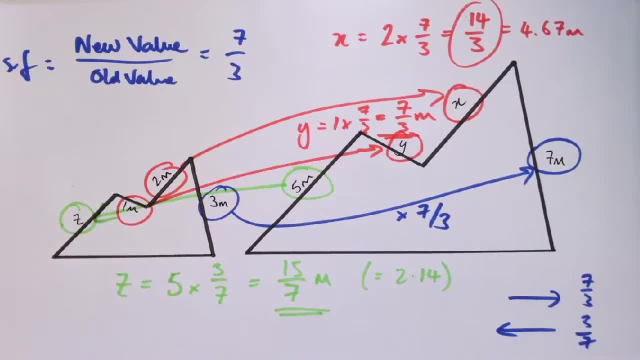 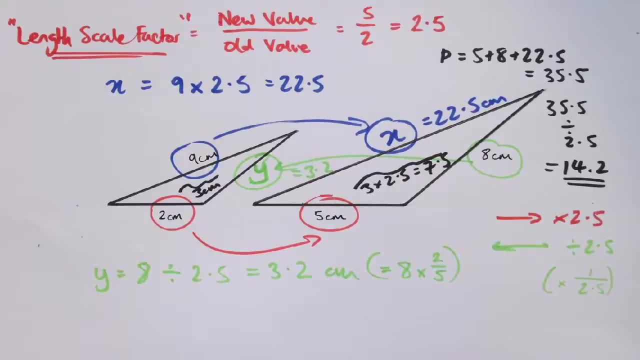 I want to get across to the idea here, which is that if you've got a length scale factor, then it applies equally to each of the different lengths between Similar shapes. The other thing we should just notice in these similar shapes is how the scale factors sort. 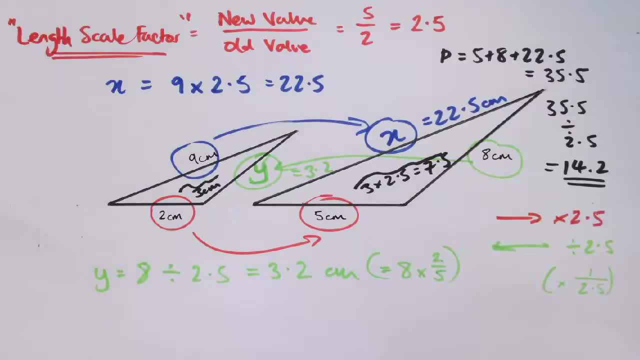 of between sides within the shapes correspond to one another. So it's not just that we've got this constant scale factor that goes from one of these similar shapes to the other, because essentially, you know, you've got the same angles, they're just different sizes. 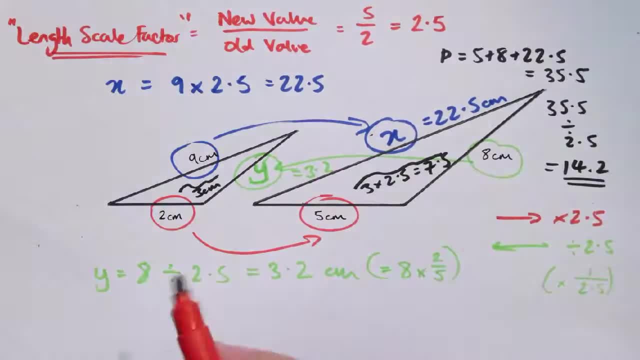 I mean strictly speaking, of course. it's not just having the same angles, It really is that one is an enlargement of the other. I could have two shapes, you know, that have the same angles, which are not similar. You know, for example, if you've got a square. 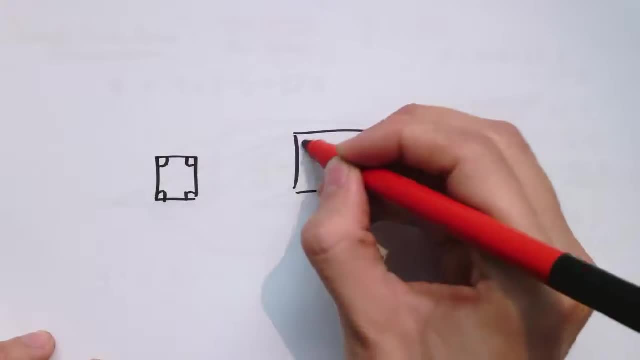 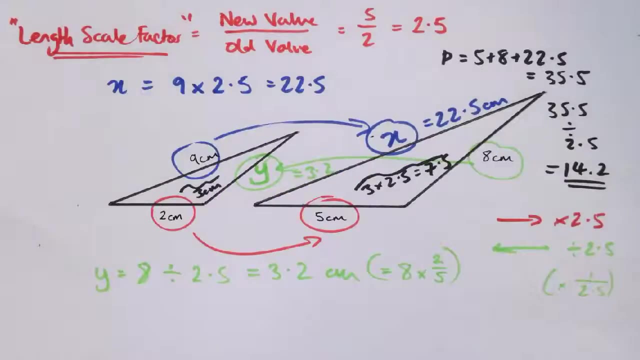 and a rectangle. they've all got the same angles, but they're not similar. But you know, but if shapes are similar, if they are just an enlargement of one another, then they'll have the same. they will have the same angles. 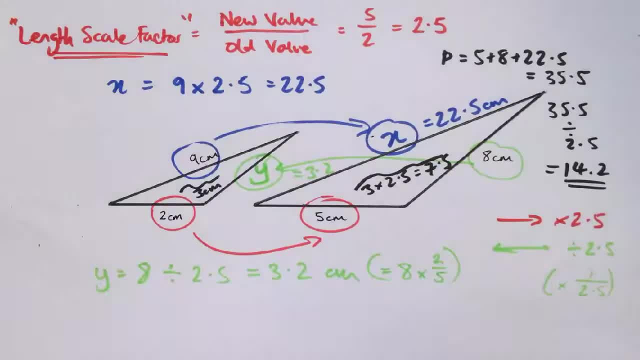 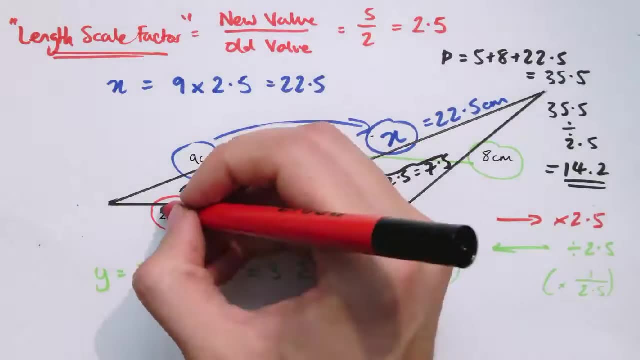 But anyway, the scale factor between sides in the shapes. So what I mean here is to say: well, look, if I take the side here 9 and the side here of 2, and look at the scale factor that takes you from. you know, 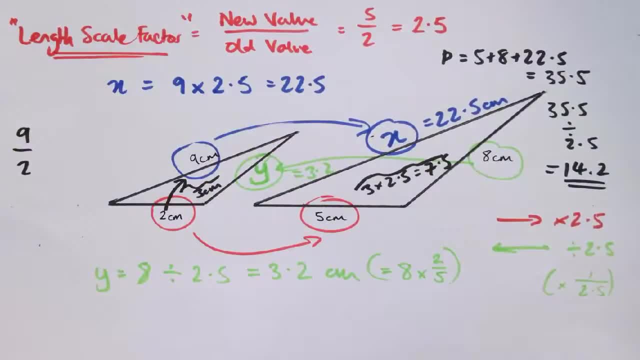 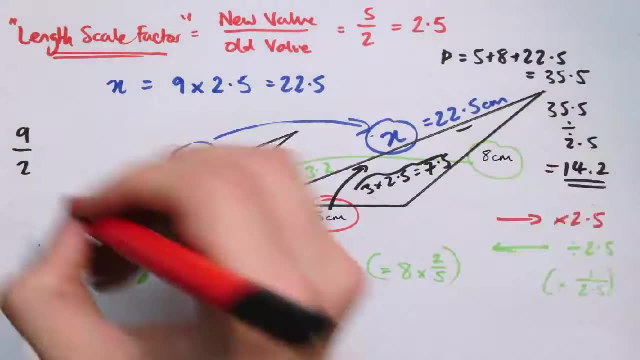 2 to 9, say that's 9 over 2.. And I look at the equivalent one in here that takes us from 5 to x, which we worked out as 22 over 5, you'll see that they are the same thing So. 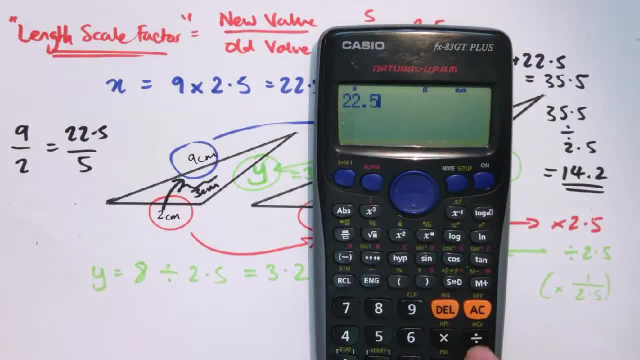 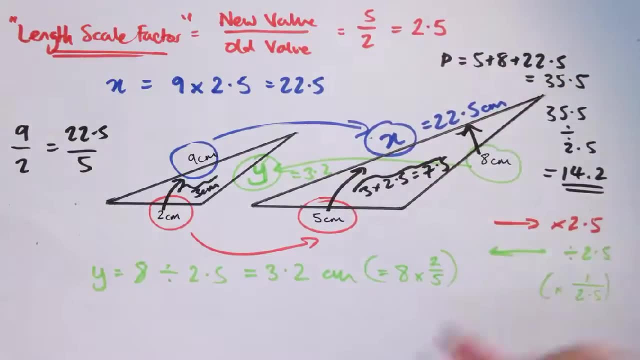 if you do 22 divided by 5, 22.5 divided by 5, you'll get 9 over 2.. Similarly, if I looked at the scale factor, that took us from you know 8 to 22 over. 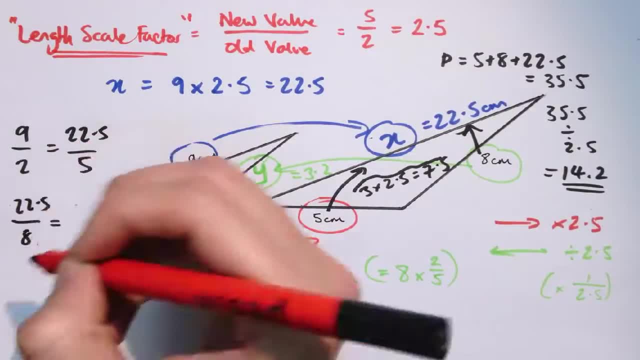 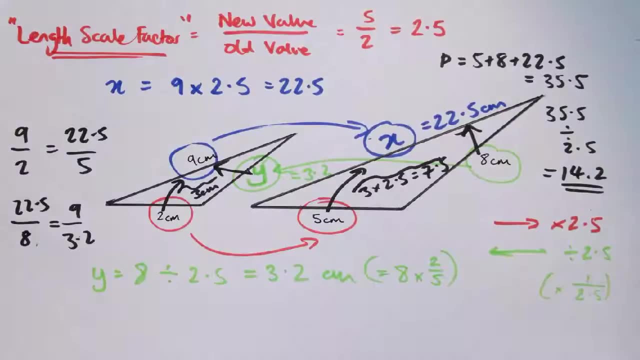 5, that would be 22.5 over 8.. That would be the same as the one that would take you from 3.2 to 9.. That would be 9 divided by 3.2. We could see we get 45 divided by 16.